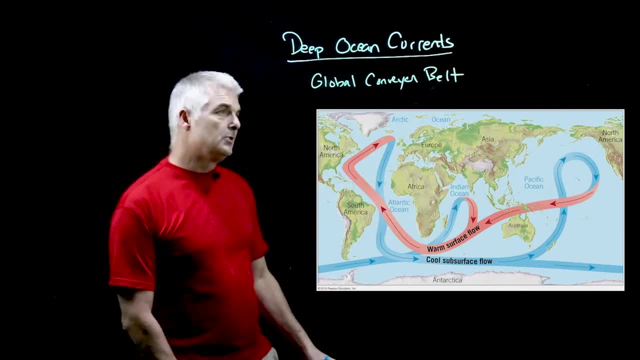 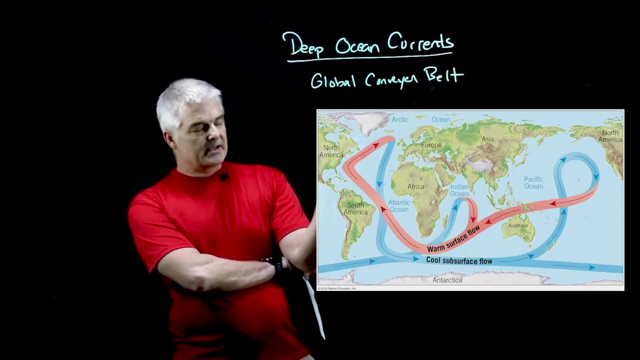 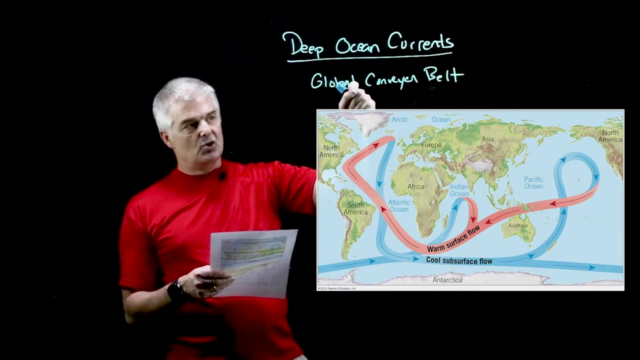 the global global, the global ocean conveyor belt and this global conveyor belt. So notice that the colors matter here- is that at the top right, When you're right up here in North America, the water sinks because it's cold, cold, dense water, which is happens at the poles here between 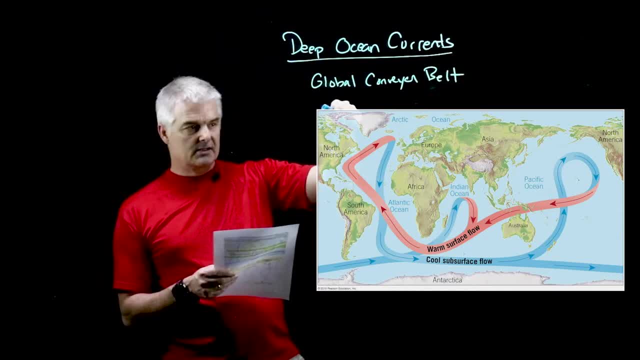 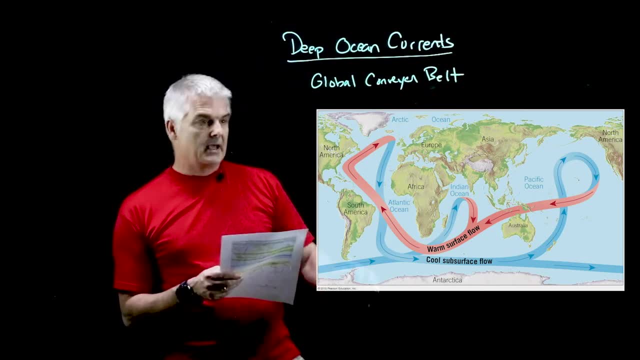 North America and Europe. And then that water sinks, and then it creates a river of water deep under the water that goes all the way through the middle of the Atlantic ocean And then, once it reaches the what did you call the Antarctica area, It zooms up and 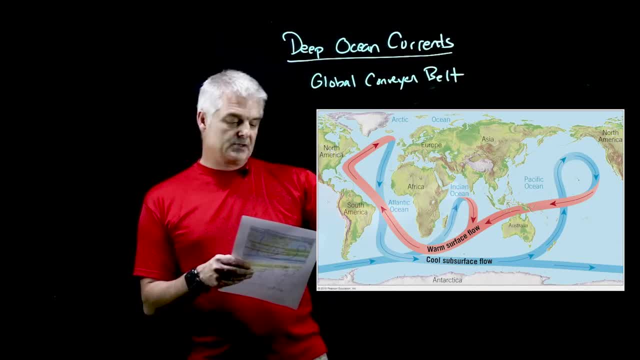 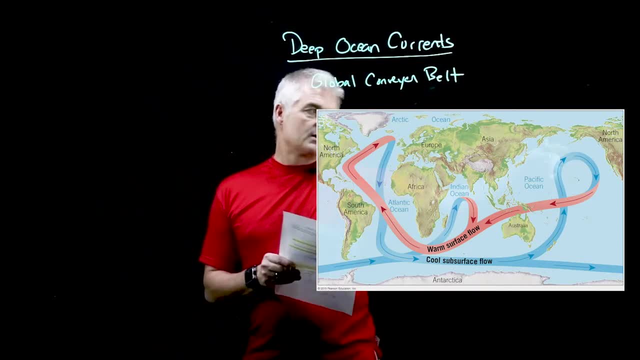 then there's kind of a split, as you can see, And then it goes up to the Pacific, etc. Now notice something I make a note in the graph is that when you get off the coast of North America over here, when it rises, it then hits warm water, All right, And then you get. 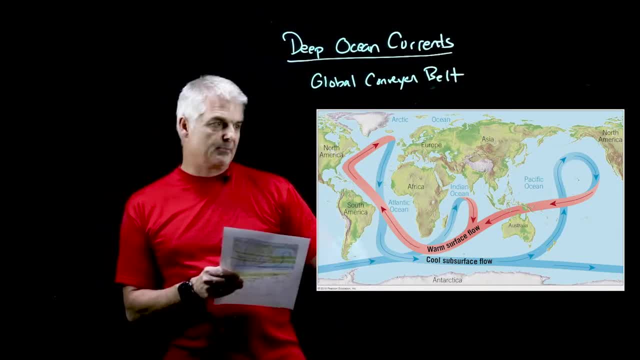 a warm surface flow. So the cool stuff at the bottom of the ocean right, And then eventually at some place it up wells, up Welling, Okay, And then it goes up to the Pacific Right. Do you notice that it does that right? Then you've got a few drops in the middle of the. 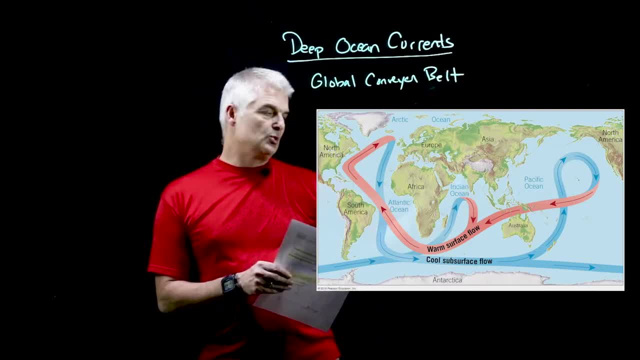 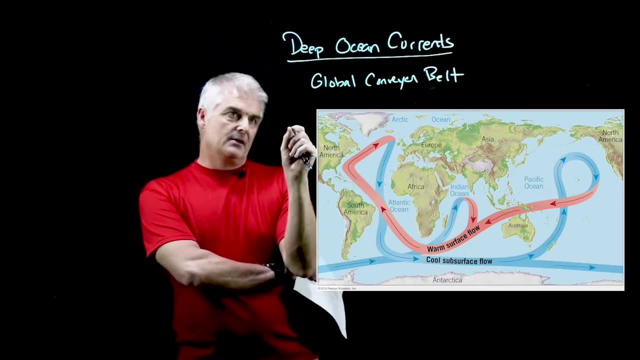 ocean right And then eventually at some place it up wells, up-welling, and then you get to the and that upwelling then creates a whole new ball game up there and then again resyncs. so there it's caused by the sinking primarily in in the polar. 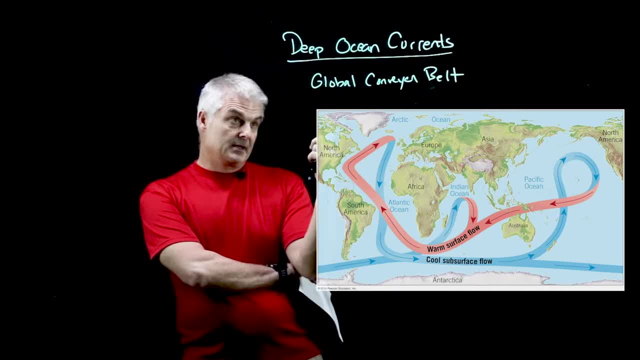 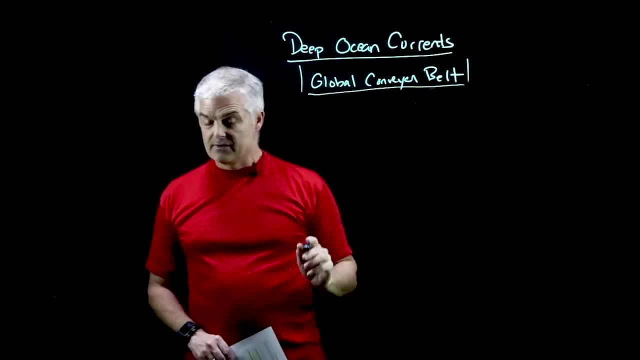 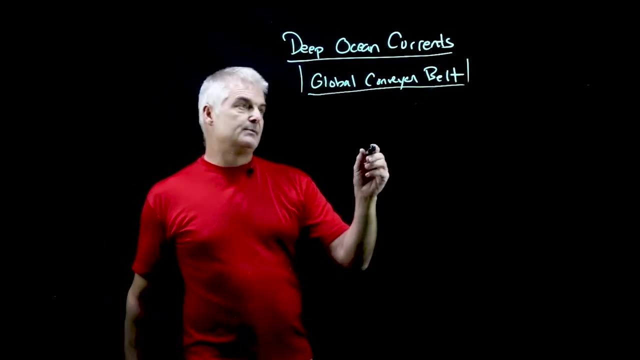 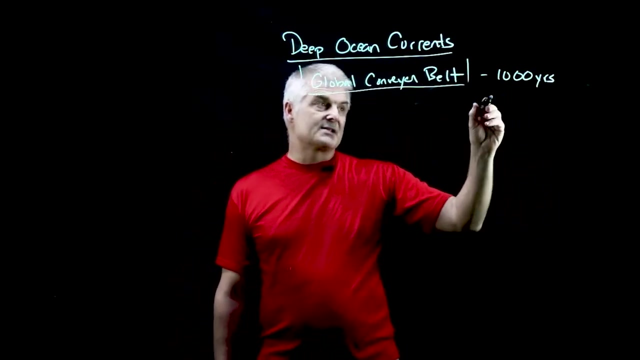 regions, note at the and kind of near the North Pole. and then it creates this crazy pattern and and this flow is not fast, though the, the surface flows can be quite rapid. this the conveyor belt. what's the number? it takes it about a thousand years for, say, one molecule to make a complete circuit. so it's not. 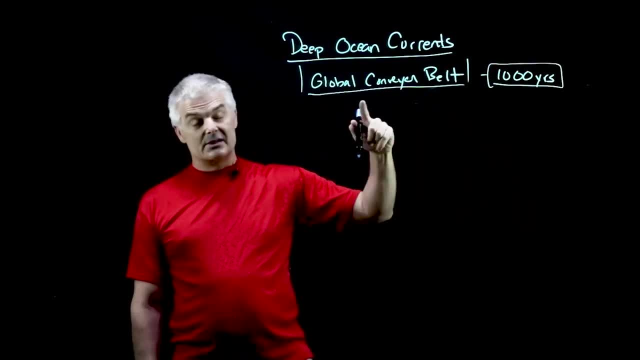 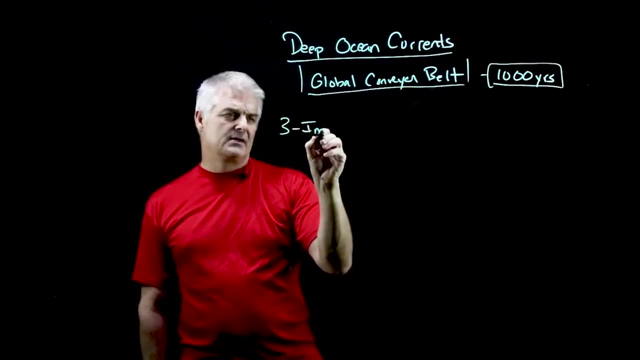 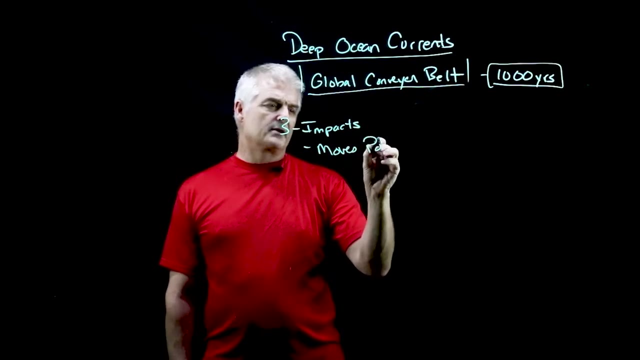